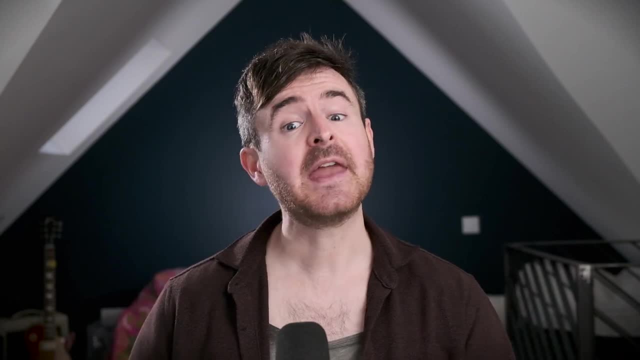 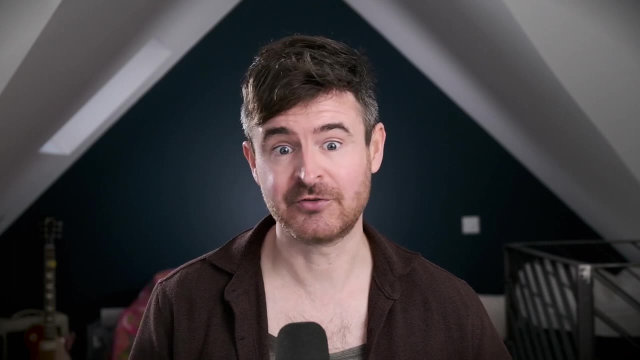 what does that mean? What is soundness, What is completeness? And then, in subsequent videos, it's going to be about how do we actually prove this stuff in relation to the proof trees that we've been looking at so far. Okay, so if that sounds good to you, do me a favour before we get. 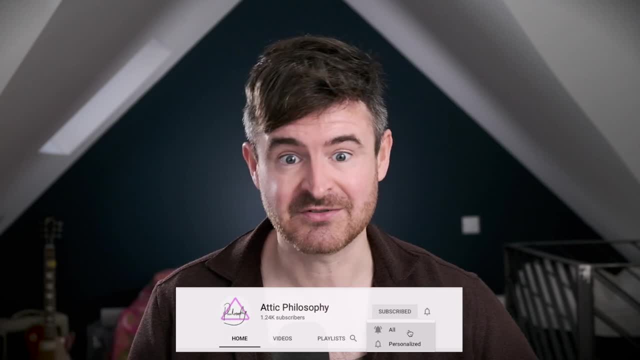 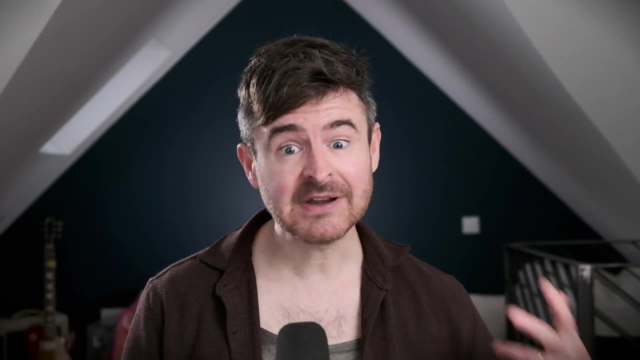 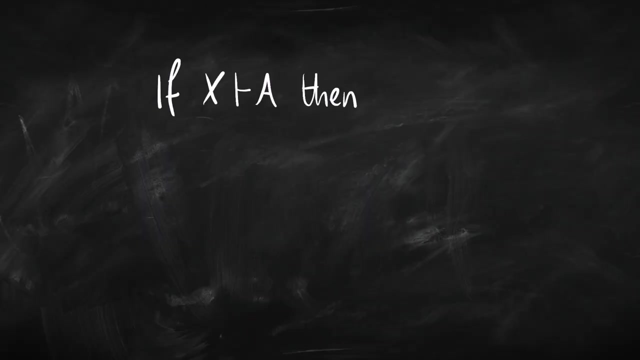 going give this video a thumbs up and why not subscribe to the channel? Okay, so when we're talking about soundness and completeness in the context of reasoning about a proof system, what do we mean? Let's take a look. So this sentence I've written here is soundness. It 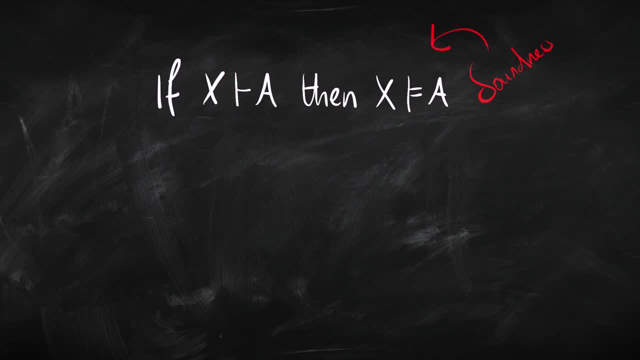 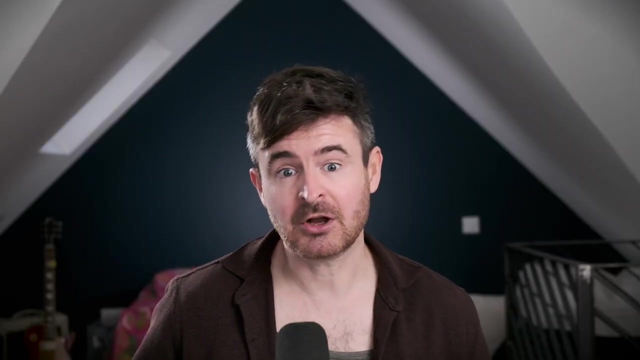 captures the idea of soundness. X here is the premises in the argument, A is the conclusion. So this is something we're trying to prove. This says that X proves A or that we can prove A as a conclusion from X as premises using natural deduction or a proof tree or whatever. 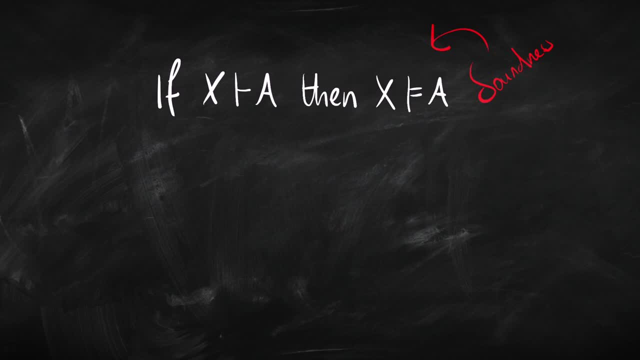 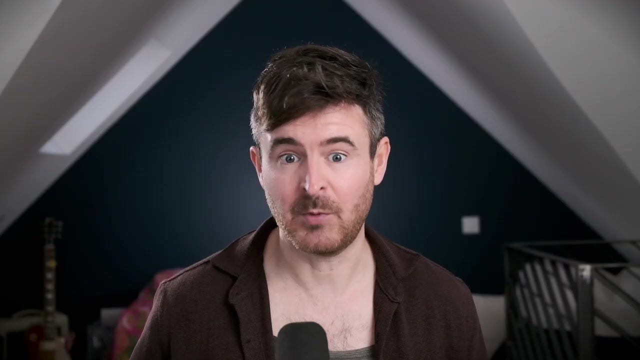 This says that A follows logically from these premises, Or that the premises entail this conclusion. Okay, so what soundness is saying is: if we prove something, then it's true, It's a genuine logical entailment. So whenever we prove a conclusion, 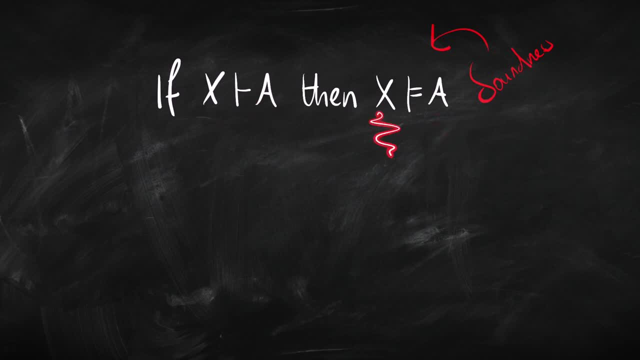 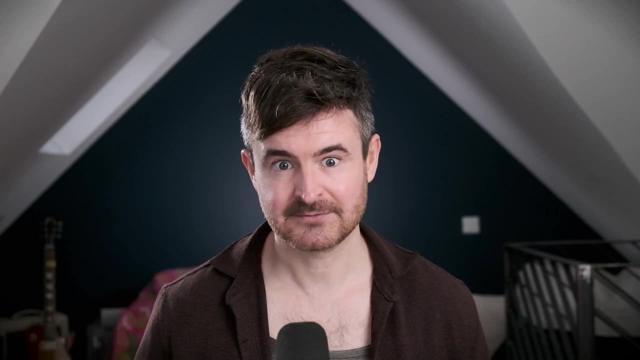 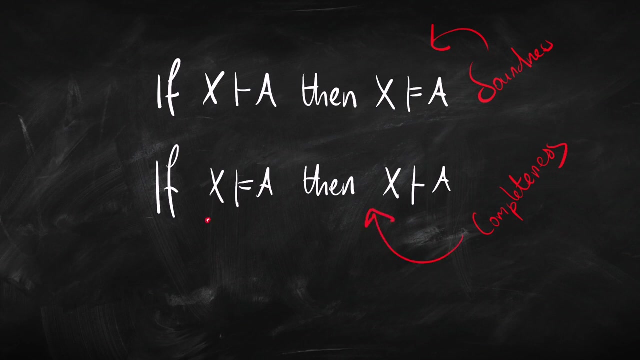 from some premises, that conclusion really does follow logically from those premises. If we prove something, then it's true. That's soundness, This statement. here it's basically going the other way around. So it says: if we've got a genuine entailment from some premises to a 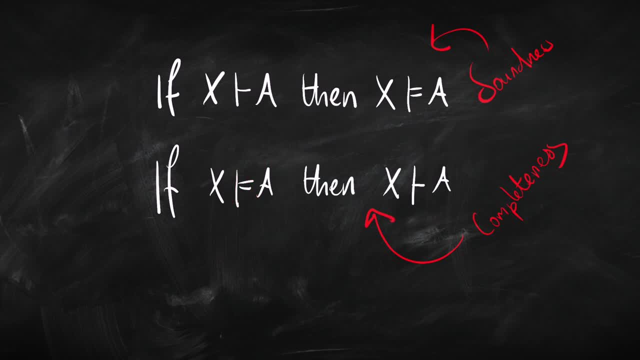 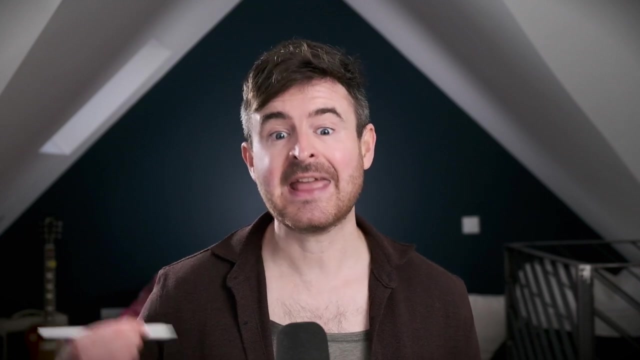 conclusion, then we can prove it. So, whereas soundness says that anything we prove is a genuine entailment, completeness says: if we've got a genuine entailment, then we can prove it. Completeness is our guarantee that our proof system does enough. It captures all the entailments. 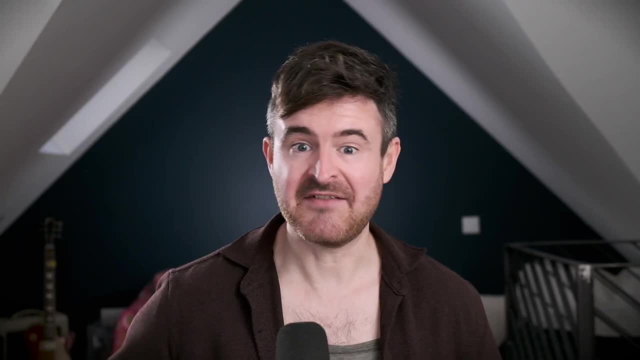 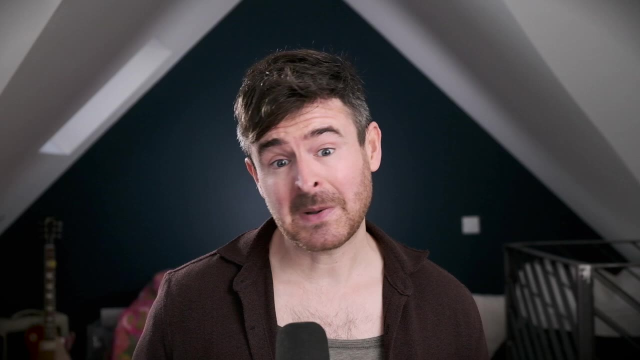 out there, Whereas soundness is telling us that if we get a result from our proof system, then it's a true one. It's a genuine entailment. Soundness and completeness: they're both important principles when we're talking about a proof system. 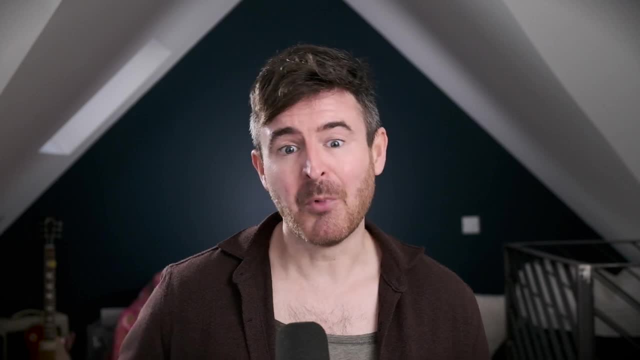 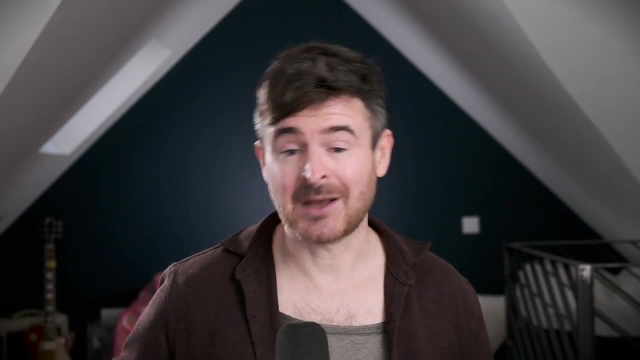 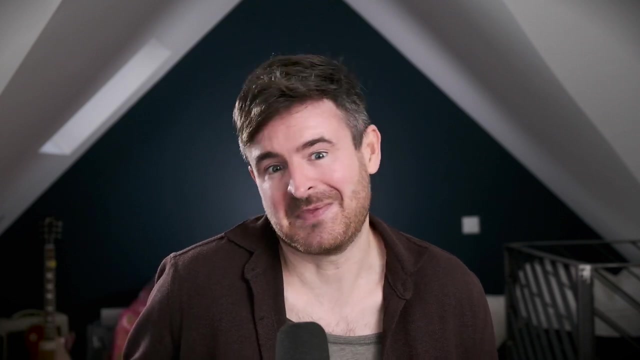 for a logic. But I guess soundness is the more kind of basic, really important principle. If you've got a proof system and it's not sound- that is, sometimes it tells you some stuff and that stuff isn't true- you kind of don't have a proof system there at all. You've got something that might just. 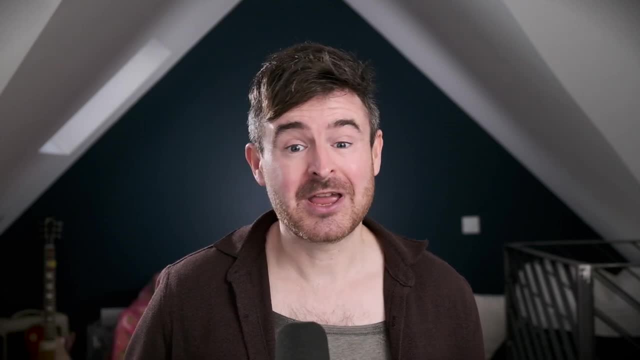 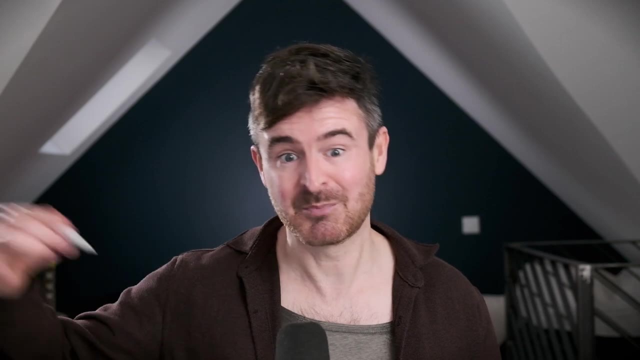 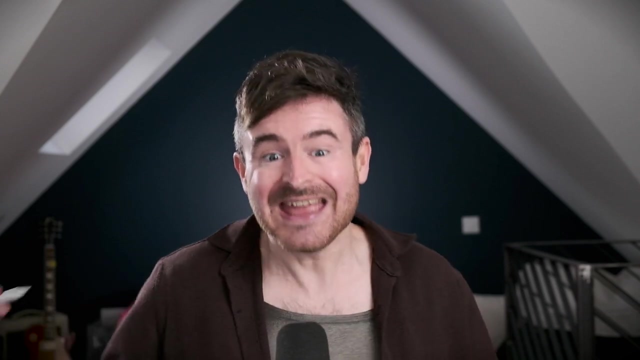 be giving you junk Right. So whenever we're talking about proving something, it's kind of part of the concept that we're proving something that is genuinely the case. If we're proving an entailment, a conclusion from some premises, it's part of the concept of a proof that it really is a genuine. 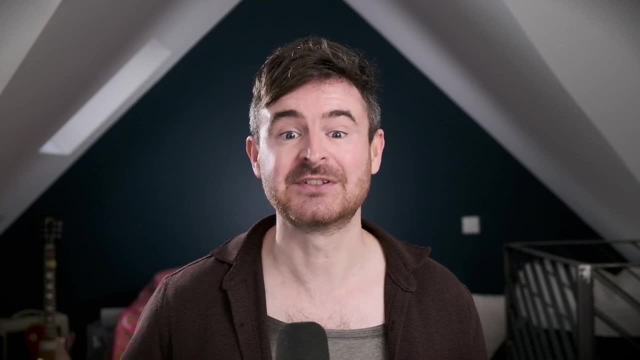 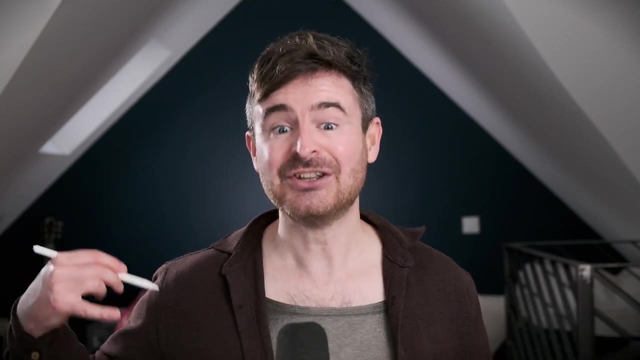 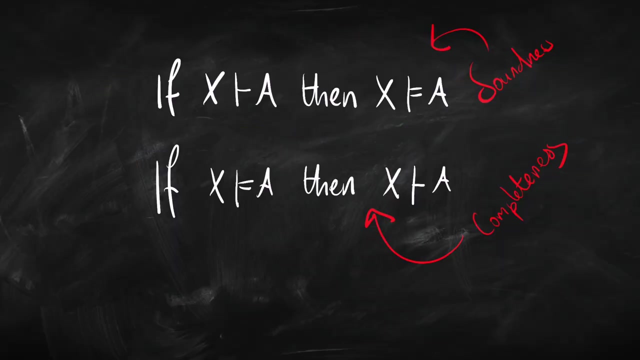 entailment. That conclusion really does follow from those premises. Okay, So soundness is our guarantee that our proof system, kind of proof in inverted commas, genuinely gives us what we're going to want from a proof. So soundness, that's kind of non-negotiable right For a good proof. 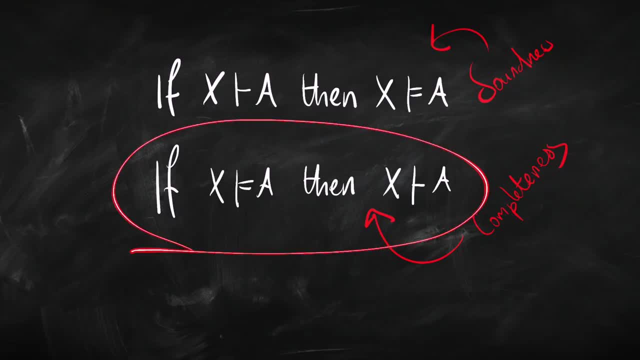 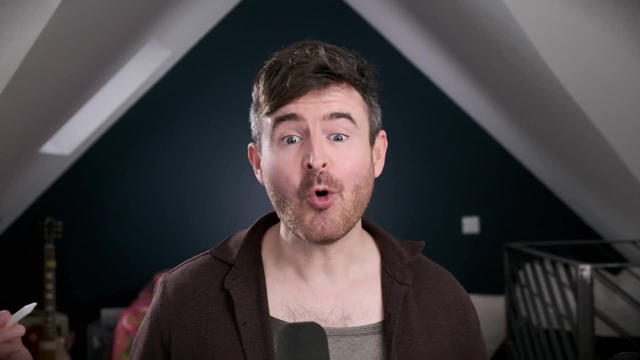 system, it's got to be sound Completeness. well, you know that's important too, but I guess it's not quite so important. So for one thing, not all logics out there are complete. That is not all. 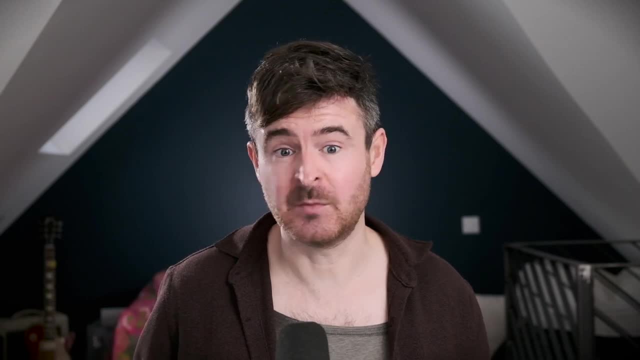 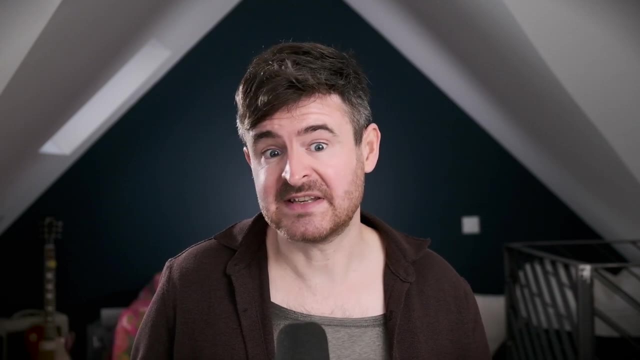 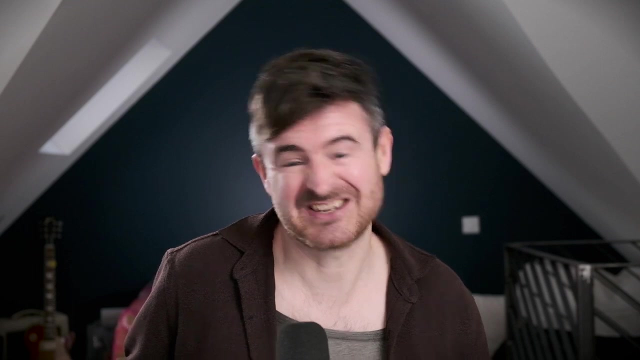 logics have a complete proof system available. Some logics so in particular classical second order logic- No complete system available for it. And a lot of people think that mathematics is kind of second order logic, It's kind of set theory. Okay, So if that's right and mathematics is, 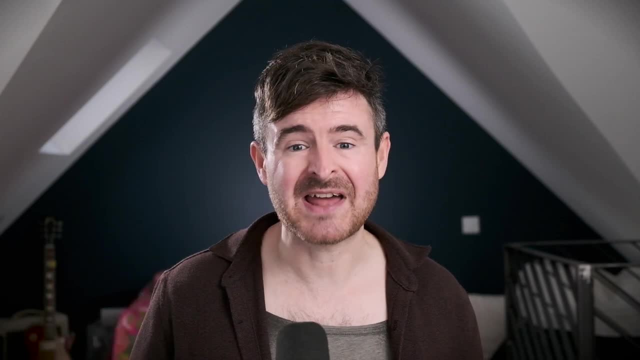 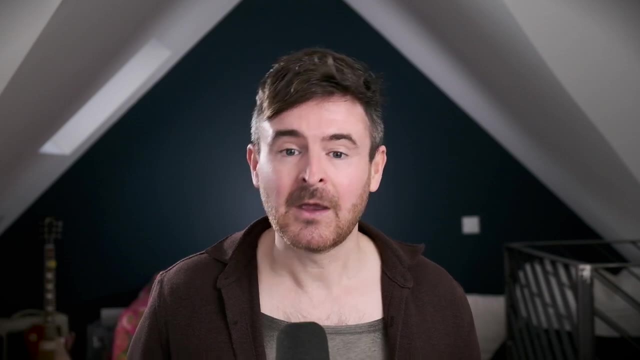 incomplete, that is, we can't prove all the truths of mathematics. Well, maybe that's not the end of the world, because we can still prove lots of them. So you might think that, yeah, in simple cases, completeness is important. 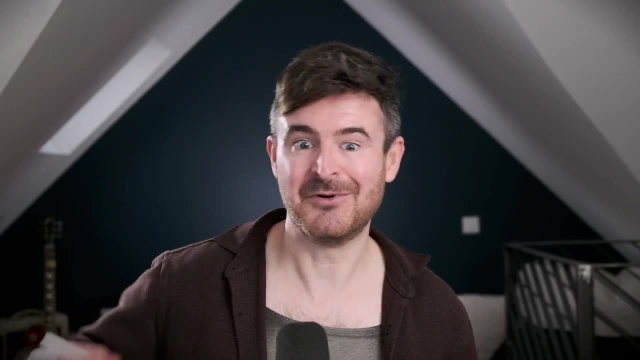 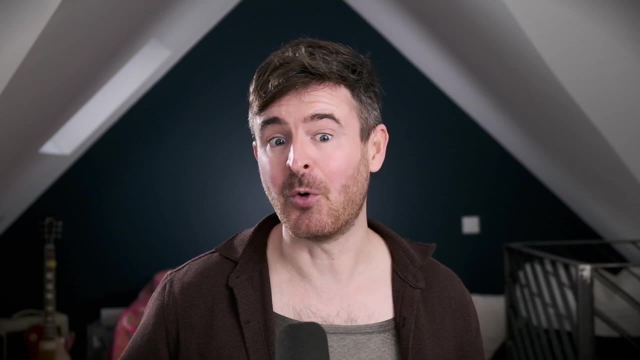 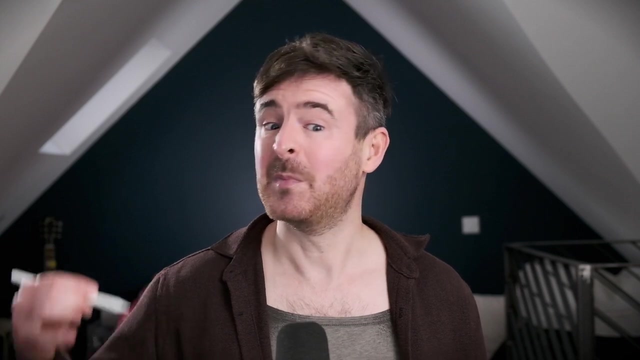 And lots of the simpler logics, logics that are simple than all of mathematics. we can prove all of the entailments in those. Okay, That's a good thing to have, But for more complicated cases where we can't necessarily prove everything, it's not the end of the world, Okay, But it is. 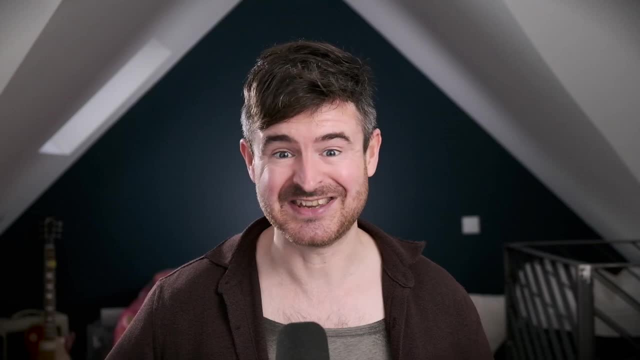 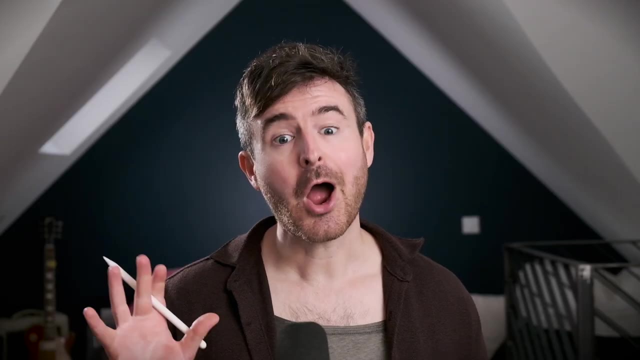 super important that any proof system we're putting forward as a good system is sound, That is, it only gives us an answer. if that answer is true, Okay, Let's go into a little Bit more detail here And let's just focus in on soundness. The same kind of stuff will go for 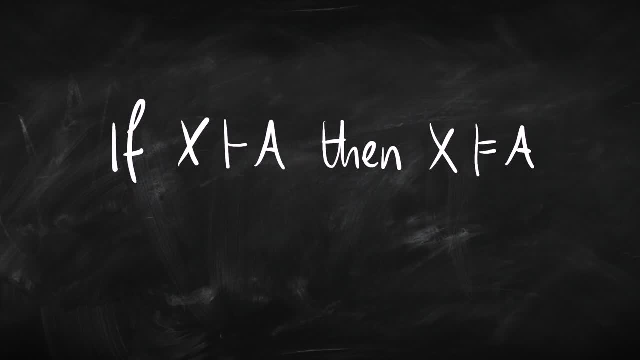 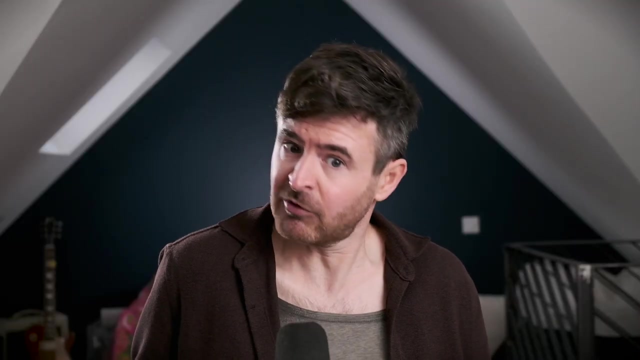 completeness. When we're talking about soundness, what are we talking about? What are we talking about here And what are we talking about here? Well, here we're talking about proof. Okay, But we've already seen that there are lots of different ways of doing proofs. There's natural deduction. 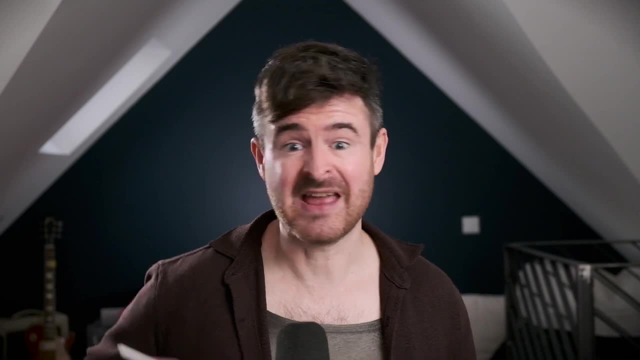 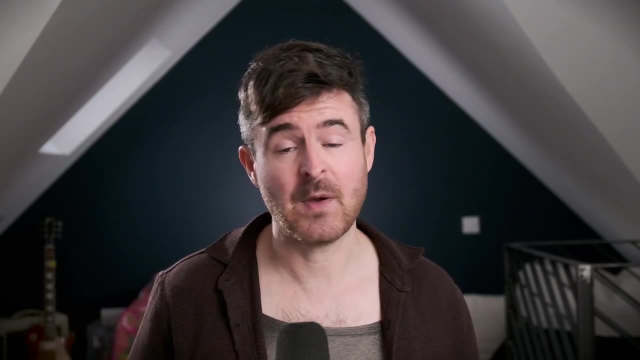 There's tree proofs, There's other systems like Hilbert proofs, There's resolution systems, There's a bunch of other stuff. We could even use truth tables if we're thinking about propositional logic. So what do we mean here? Well, it depends, right. 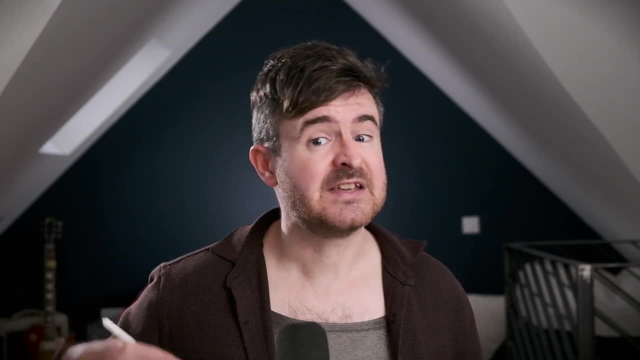 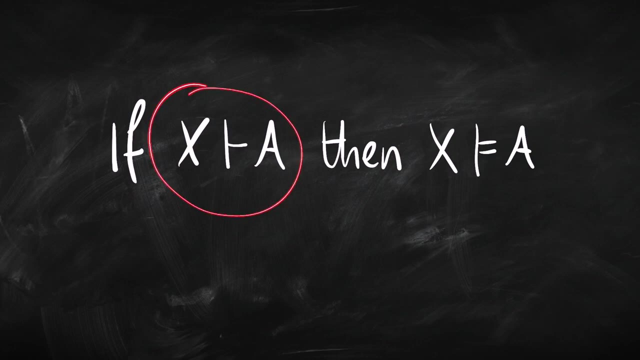 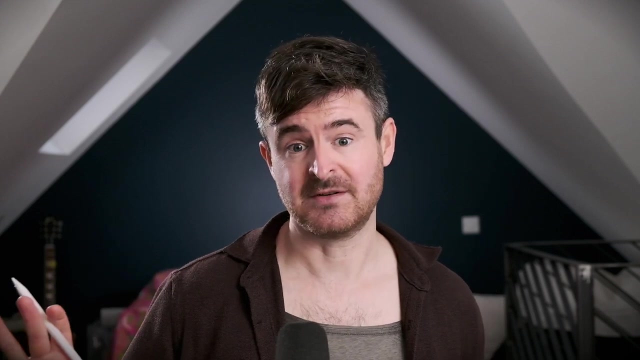 We're not talking so much about soundness or completeness in general. We're talking about a particular proof system. Okay, We're talking about the tree test or a natural deduction system or whatever. So we're going to be saying, oh, this proof system is sound, or this proof. 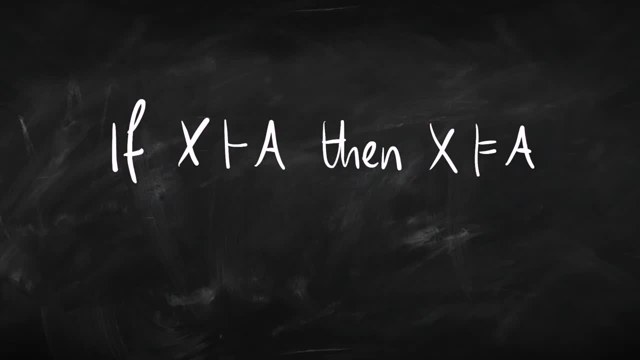 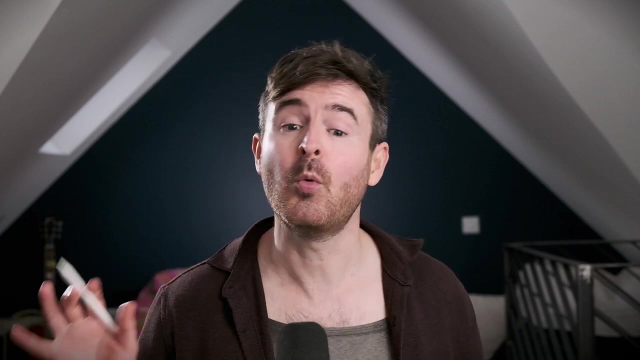 system isn't sound Over on the right. here we're talking about entailment in a particular logic. Okay, So this might be classical propositional logic. It might be classical first order logic. It might be some other more exotic logic, It might be relevance logic or whatever. 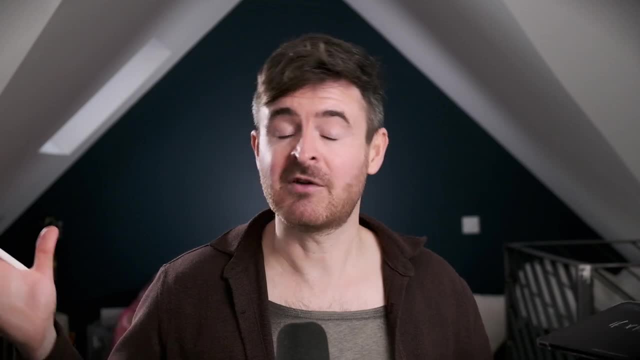 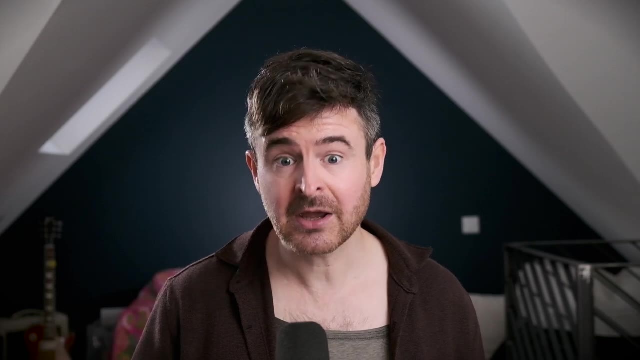 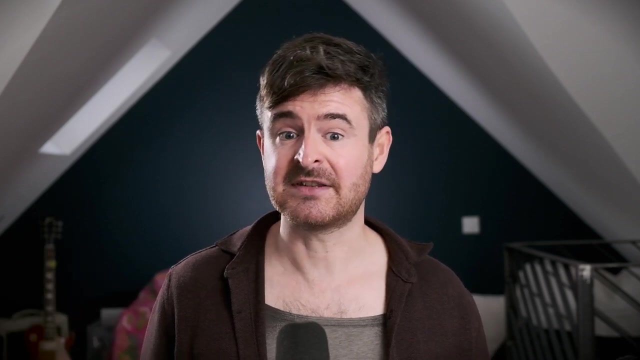 So there's kind of two extra parameters that are involved. when we're talking about soundness or completeness, We're talking about a specific logic and we're talking a specific proof system for that logic. So we might say, for instance, that the 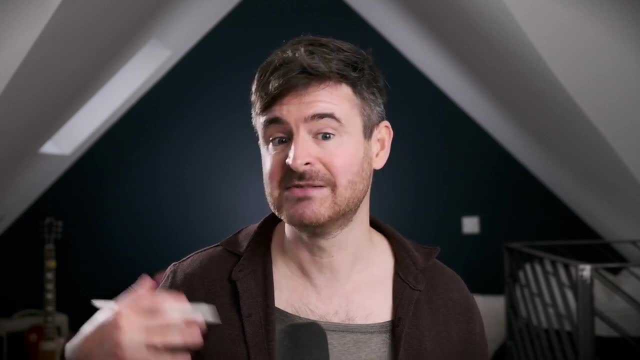 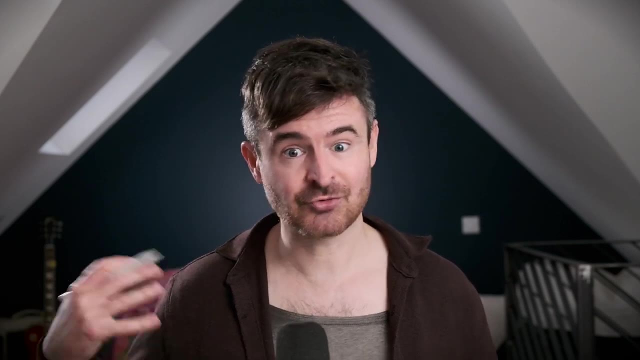 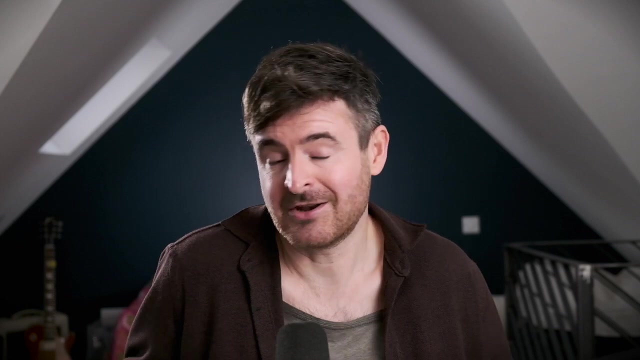 truth table test is a sound system for classical propositional logic. That's true. We might say that the tree system of proofs is a sound system for classical first order logic. Okay, Given the kind of trees. Yeah, that's true. Sometimes you'll hear people talking about completeness. 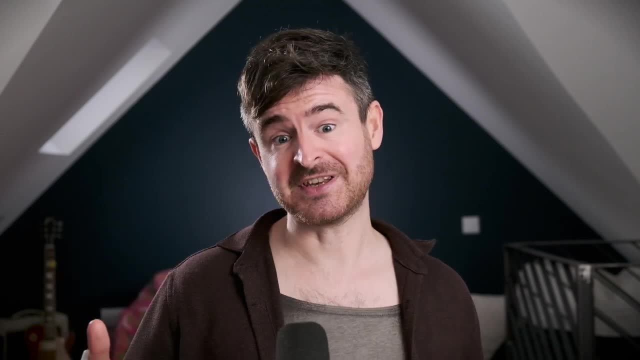 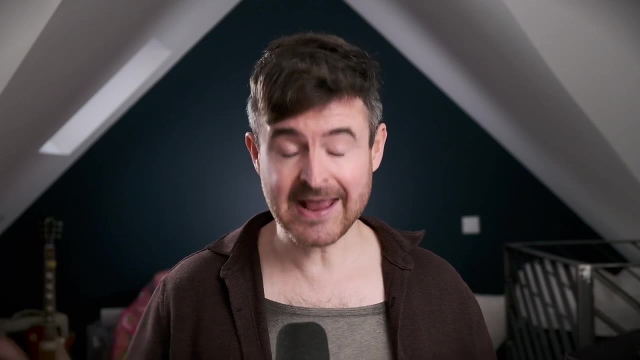 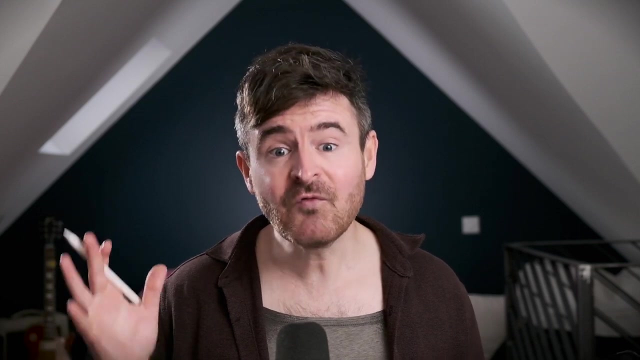 or incompleteness of not a particular proof system, but of a logic in general. Okay, So earlier on I said that second order, classical logic is incomplete. You've got Gödel's famous incompleteness theorem, Whereas you might say that classical, first order logic is complete. 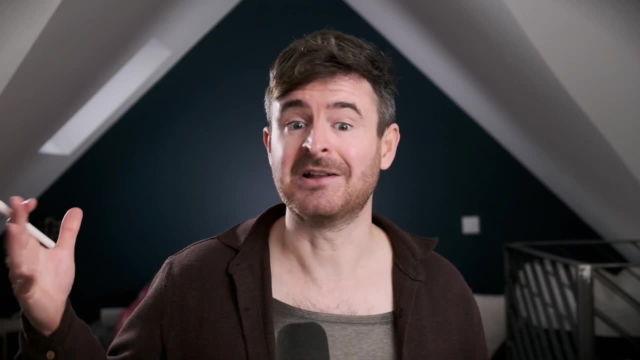 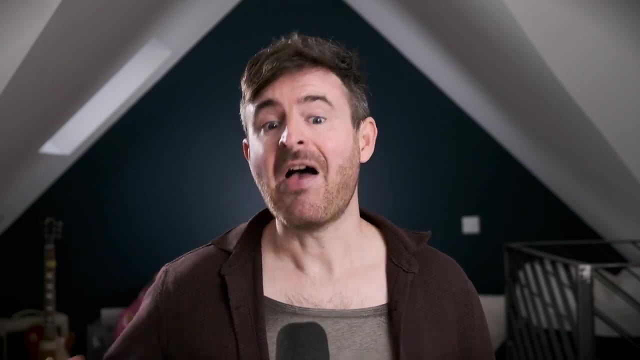 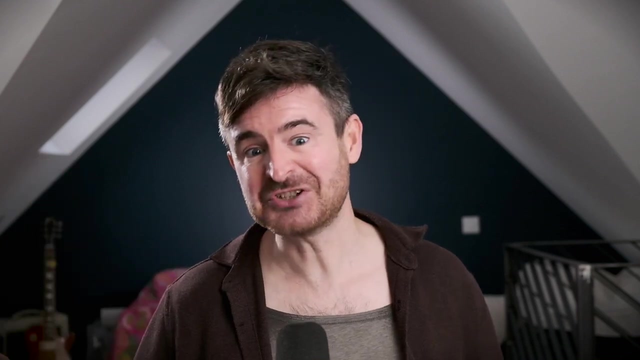 So there, I haven't mentioned any particular proof system. I've just said that these logics are complete or incomplete. What does that mean? Well, to say that a logic is complete kind of means that there is some proof system available for it. Okay, So a complete logic is kind of like.